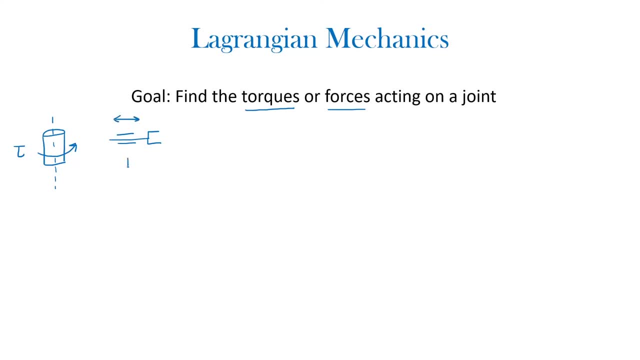 simply move linearly up or down and therefore would have a force acting on it. So what you have to know is that if you have a revolute joint, you would calculate a torque, But if you have a prismatic joint, you would find a force. 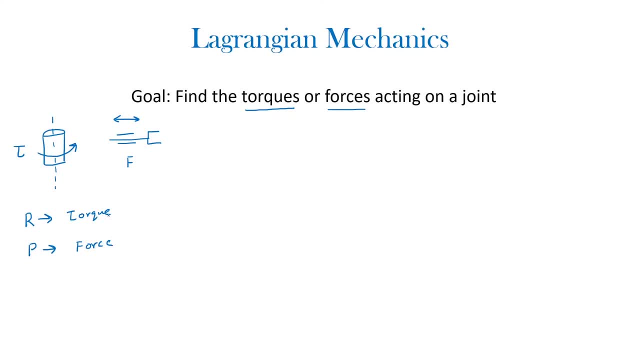 Right Now the torques and forces can be found using the Lagrangian. The Lagrangian, simply denoted by the capital letter L, is equal to the kinetic energy of a system minus the potential energy. So as a shorthand notation I will just use the Lagrangian function. So if you 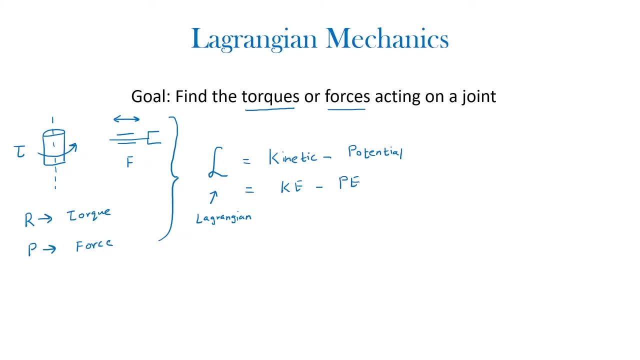 use Ke for kinetic energy, minus Pe for potential energy. Now the terms for kinetic and potential energy would exist in terms of whatever variable is used in the equation. so, for example, you will have theta and theta dot, where theta would represent the position of the robot manipulator and theta dot 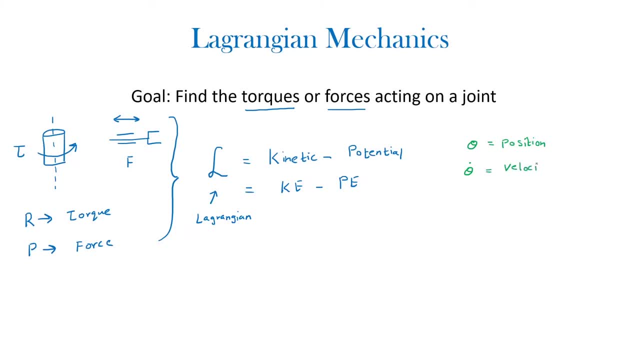 represent the velocity of the robot manipulator. So these two terms would be used to make up the equations for the kinetic and potential energy. So to find the kinetic energy we will use the equation we've been using all along, which is half m v squared. So this v? squared term will actually contain theta dot and 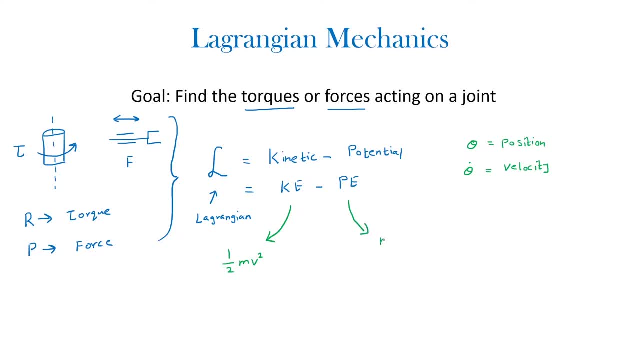 the potential energy would simply be mgh, where the height term would contain theta, which is the position. So once the Lagrangian has been calculated, we can then find the torques or the forces acting on the joints of the robot, and to do that we can simply use this equation. 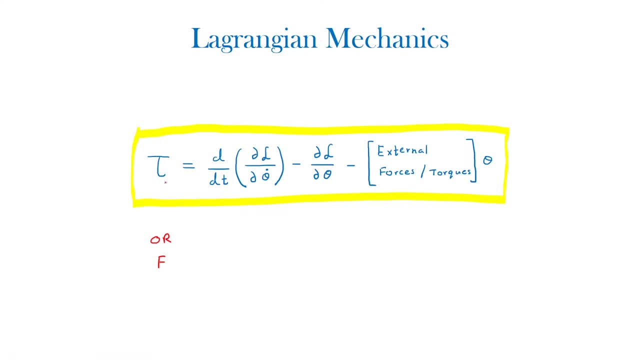 Right, so I've just used Tau here to represent the torques, but it can also be for forces. You would start off by finding the partial derivative of the Lagrangian with respect to theta dot, which is the velocity, and then finding the time derivative of that particular equation. 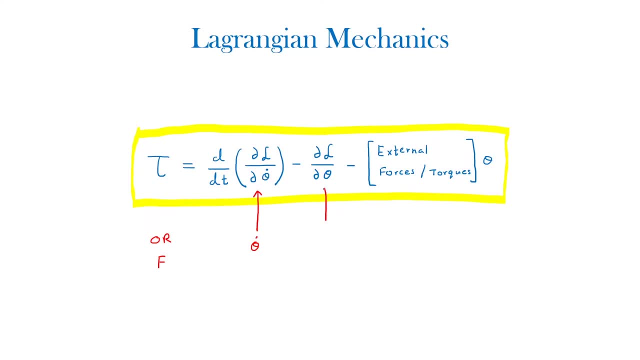 You would then subtract the partial derivative of the Lagrangian with respect to theta and finally subtract any external input, torques and forces- and that would be multiplied by theta. So the overall steps that you would follow when solving a problem involving Lagrangian mechanics. 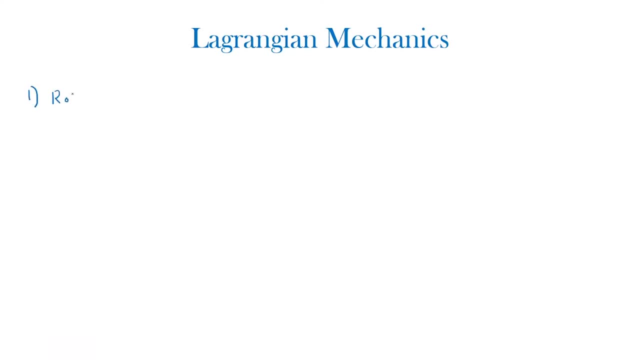 would be, first of all, to analyze the robot system or the robot manipulator, And from this you would be able to find the position vector of the joints or whatever parts you're looking at. And that would be the position vector of the joints. 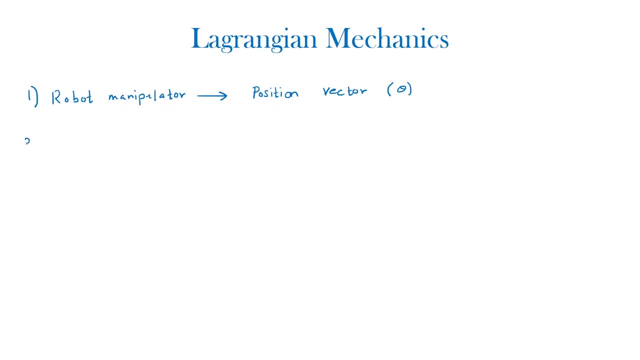 And that would actually be represented by theta. You can then differentiate the position vector, And by differentiating it the velocity vector can be found. Now, the velocity vector would be represented by theta dot. We can then use the position and velocity vectors to find the kinetic energy. 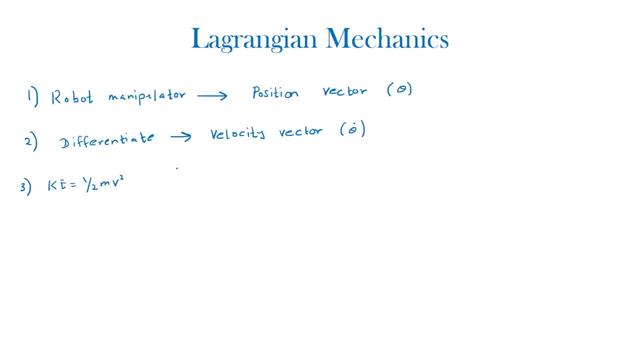 which would be half n. So that would be mv squared, where v is the velocity vector and the potential energy, which is simply mgh, h including the position vector. We can then use the kinetic and potential energies to find our Lagrangian. 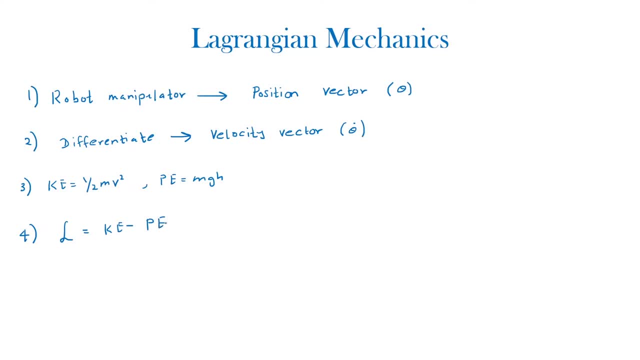 which is kinetic energy minus the potential energy. And once we have found the Lagrangian, we can then find any torques or forces acting on the joints using the equation we discussed in the previous slide, Which is this equation And any external inputs. 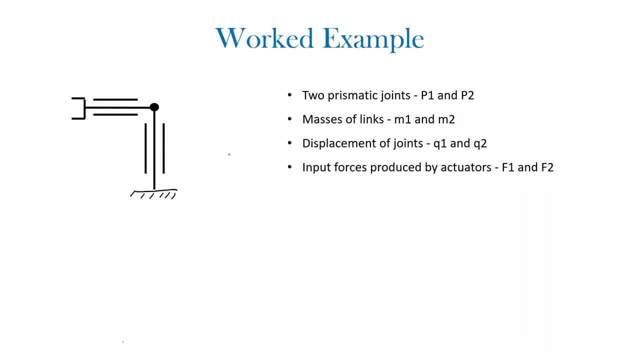 Right. So to make things clearer, let's go through a worked example. This is the Lagrangian. This is the Lagrangian. This is the robot under question that we will be looking at. So it has two prismatic joints, first joint being P1 and the second joint being P2.. 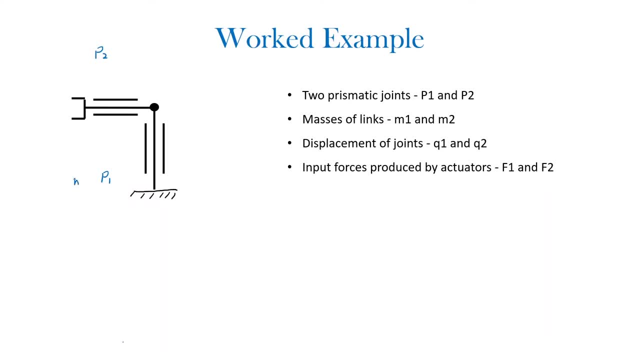 So P1, the link attached to joint P1, has a mass of m1.. And the link attached to P2 has a mass m2.. There is also some displacement as they are prismatic joints. So P1 can actually move linearly upwards and downwards and it will do so with displacement q1. 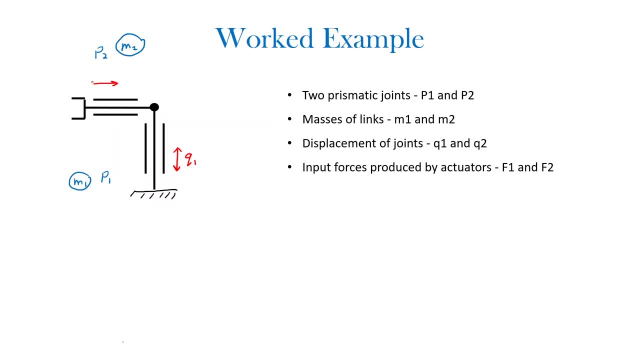 So P1 can actually move linearly upwards and downwards, and it will do so with displacement q1. While P2 can move from side to side with displacement q2.. While P2 can move from side to side with displacement q2.. In addition, there is an input force acting on each joint. 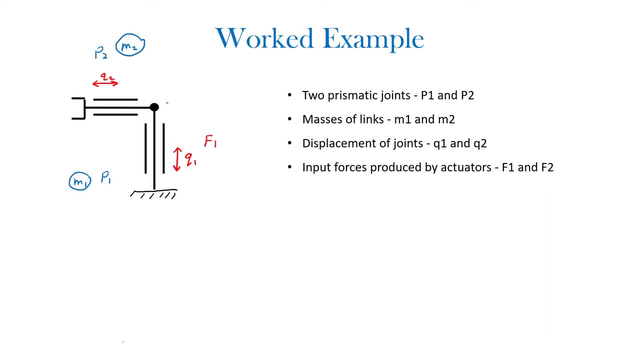 So for the first joint we have an input force of F1.. And for the second joint we have an input force of F2.. So the first step in solving this problem would be to find the position vectors of each of the two joints. 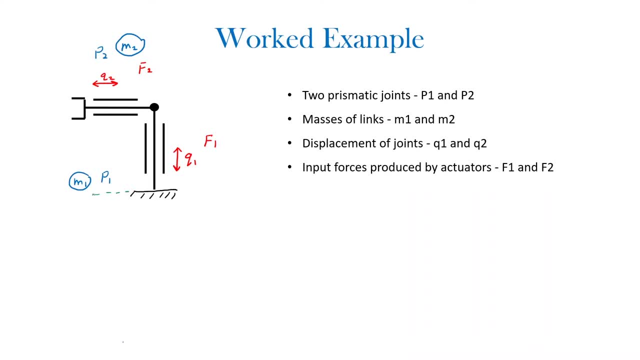 And to do this, it would be helpful to have a coordinate axis or a coordinate system. So we can imagine this as a coordinate system, so we can imagine this as our positive x-axis, and this direction would be our positive y-axis, right? so, first off, we will find the position vectors. 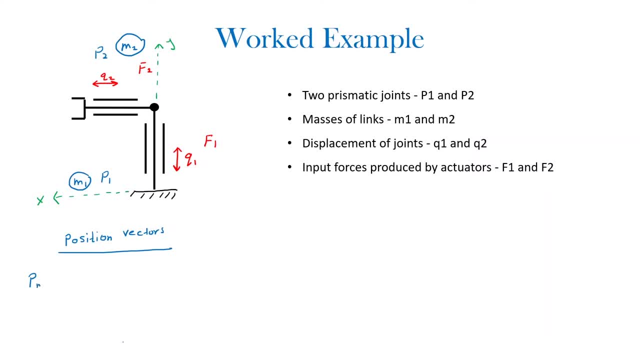 right. so the position vector of m1 can be represented as a 2 by 2 matrix. you have the x direction and the y direction. so if you look at link one or joint one, it's on the zeroth part of the x-axis. therefore it would have zero x movement. however, it can move linearly up and down, which is 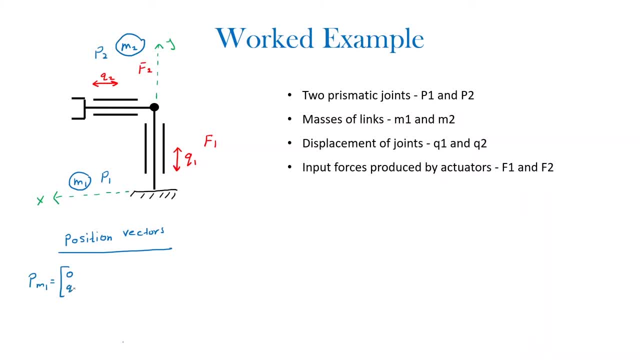 along the y-axis. therefore it can move by x, q1- sorry, q1- along the y-axis. similarly, we can also find the position vector for mass m2. it would already have a y displacement of q1, depending on how p1 moves. so therefore the y component will be q1 and it can move. 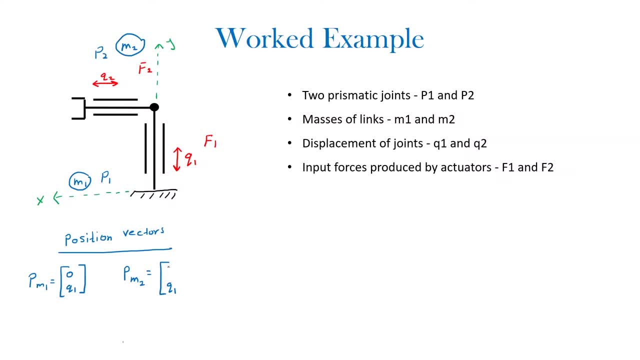 side to side by displacement q2, so it would have x component of q2 right. the next step would be to differentiate the position vectors to find the velocity vectors right. so just to clarify, the velocity vector- we can call it vm- would be equal to the differentiated version of pm with respect to time. 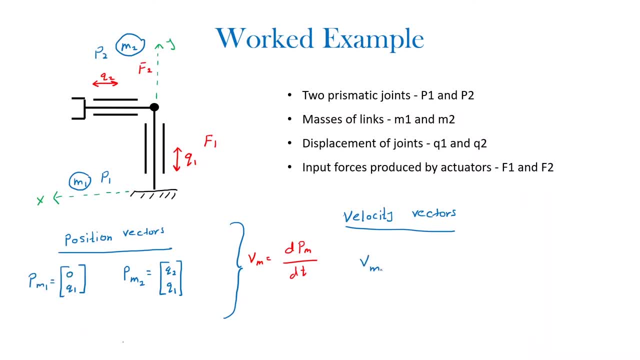 so, with that in mind, we can have v m1, which would be 0, and q1 dot. similarly, vm2 would be q2 dot and q1 dot. this is because q1 and q2 are not constants, and so they become differentiated when you are finding the velocity vector. 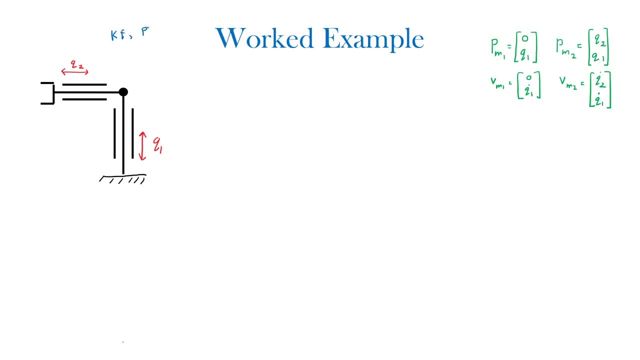 so now we can calculate the kinetic energies and the potential energies of the system. let's first have a look at the kinetic energy now. the equation for finding the kinetic energy is half mv squared, but the velocity vectors have an x component and a y component. therefore we have to consider each component separately. so we would actually have the equation. 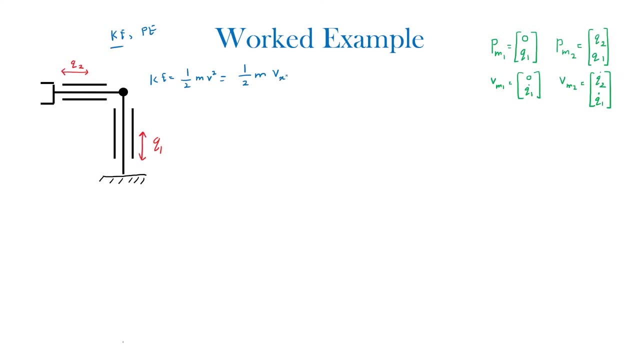 looking like: half m the x component, vx squared, plus half times mass times the y component squared. so this can be simplified to an equation such as: half m vx squared plus vy squared should be the kinetic energy, right? so with this in mind, we can now find our kinetic energies of the system. so i will use a different color. so 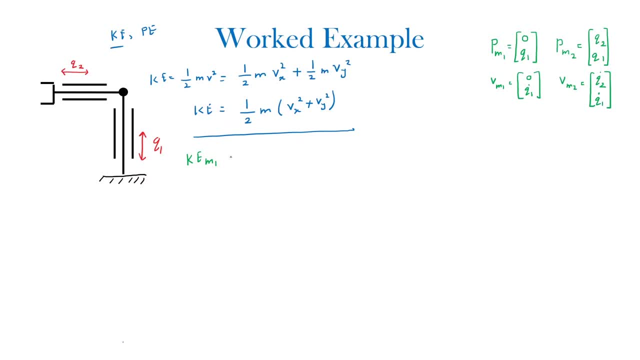 let's say kinetic energy for m1 would be half times m1 times. so vx component would be zero. so that's zero plus vy would be q1 dot. so it would be half m q1 dot squared. similarly we can find the kinetic energy for mass m2, which would be half times m2. 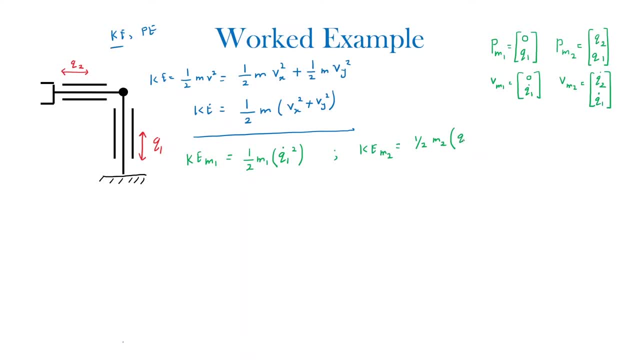 times. the x component is q2 dot, so you would have q2 dot squared plus. the y component is q1 dot- q1 dot squared, right. so the next step would be to find the potential energy of the system right. so the potential energy would be m g, h. now keep in mind that h here. 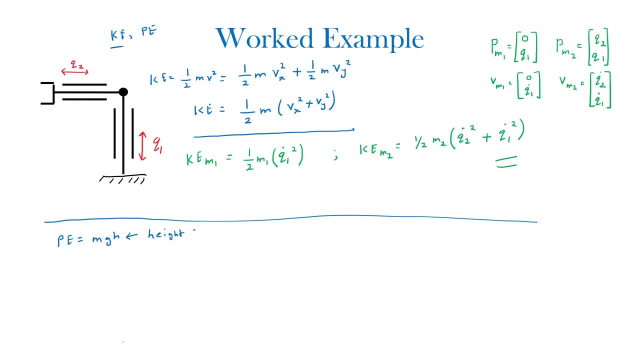 is the height, which means we only look at the vertical component when we take in the thermal energy of the system right. so the potential energy of mass m1 would be m1 g and the height or the vertical displacement would be q 1.. similarly, the potential energy for mass m2. 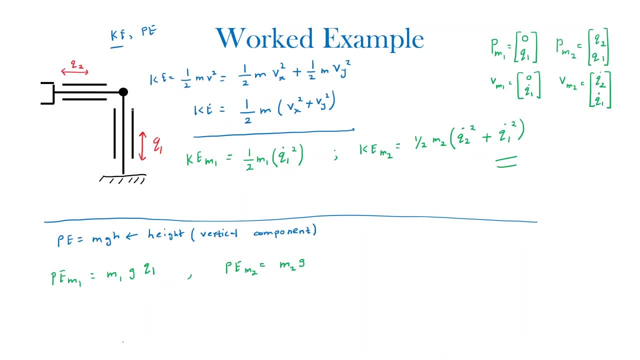 would be m2, g and the height of this would also be q1, as it only moves linearly, only moves horizontally, with displacement q2 but is at a height of q1, so it will be m2g, q1, right. so now we have both our kinetic and potential energies, for both our masses or both. 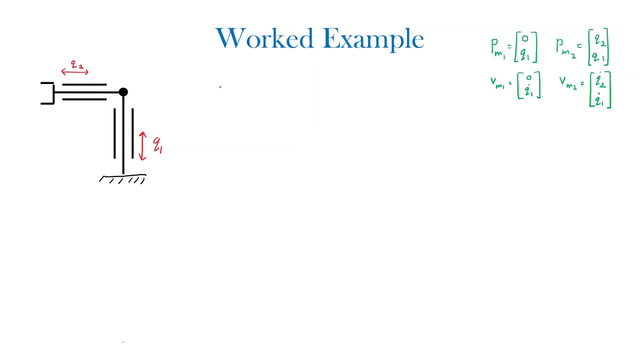 our links. so now that we have the kinetic and potential energies, we can calculate the lagrangian. it should be equal to the total kinetic energy minus total potential energy. so for our system you would have kinetic energy of m1 plus the kinetic energy of m2, minus the potential energy. 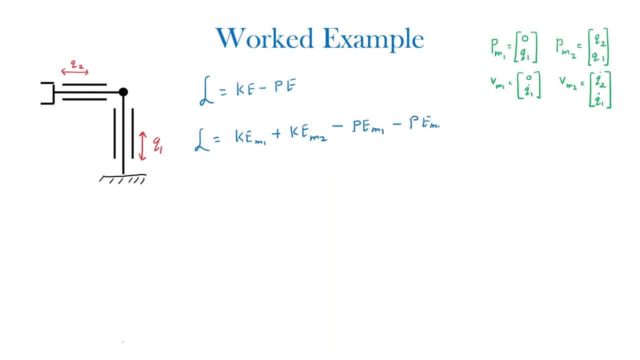 of m1 minus the potential energy of m2, and if you substitute in the terms, you would get this as your lagrangian. and if you factor out the masses of m1 and m2, you would get this as your final equation for the lagrangian. 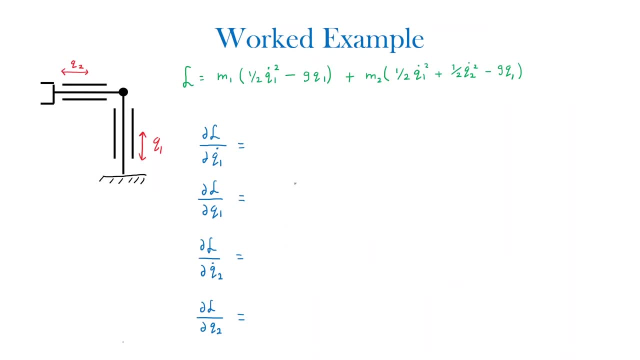 you right. so now that we have our lagrangian equation, we can find the torques and the forces. but before we calculate the torques and forces we would have to find the individual components of that main equation. so we would have to find the partial differentiation of the lagrangian. with respect, 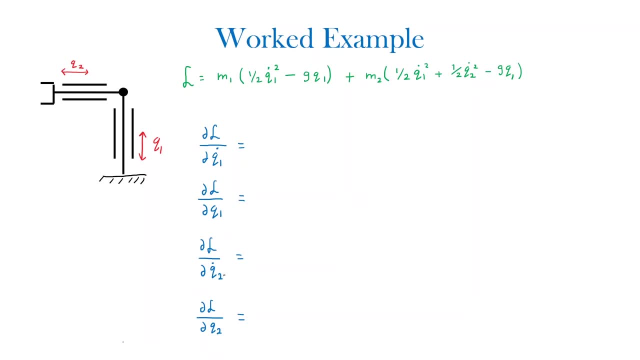 to q1, dot, q1, q2, dot and q2. so the final step would be to calculate the torques, or forces, now that both our joints are prismatic. therefore, we would be finding two forces. we can call them fm1 and fm2. the equation we would be using would be this equation. so, for example, 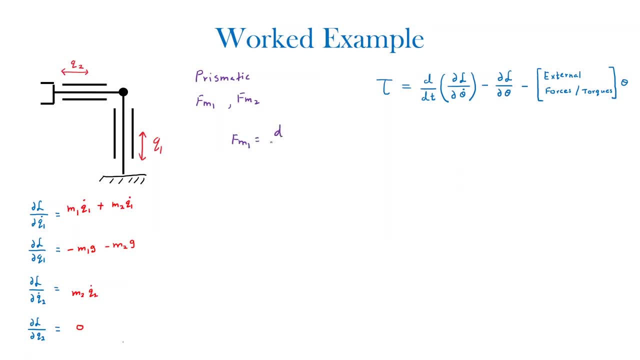 fm1 would be equal to the time derivative of daba l over daba q1, dot minus daba l over daba q1, minus any external input forces and torques. we had an external input force which was f1 times q1 right. similarly, fm2 would be equal to d over dt. 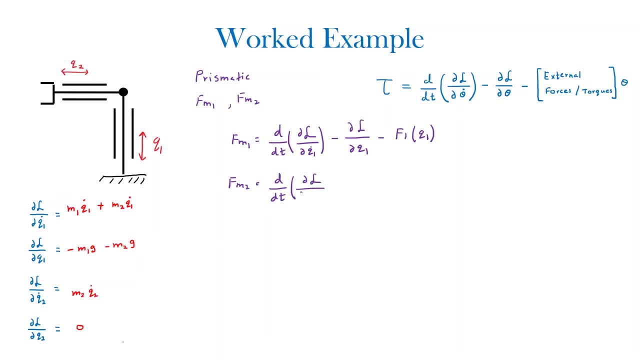 partial differentiation of the lagrangian with respect to q2 dot minus daba l over daba q2 minus the second input force, which was f2 times q2, right? so if you were to substitute in the values and solve for this, you would get these two equations. now i didn't solve this part over here. you can actually leave. 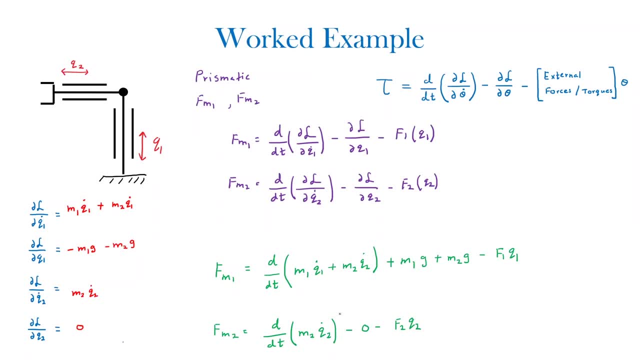 your answer like this: if you want, but if you want to solve it, for example this part over here- the time derivative would simply be m2, q2 double dot, and this q2 double dot would actually be the acceleration of that particular label. so this is your final answer. 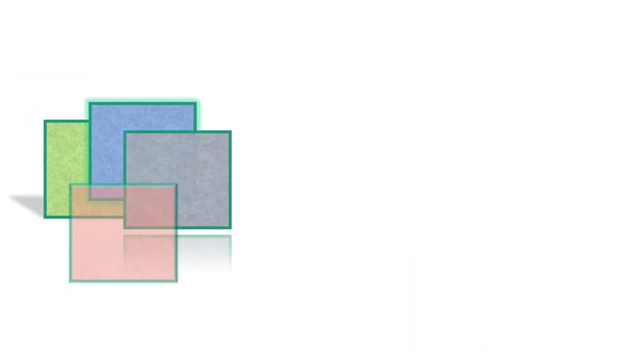 all right, guys. so that's all for this video. i hope you guys learned something and enjoyed the video. if you guys like the video, don't forget to give me a thumbs up by clicking the like button and if you haven't done so already, please hit that subscribe button now. if you have any questions or 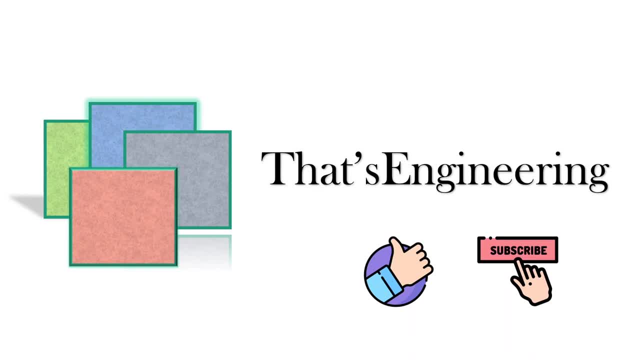 clarifications on the grandian mechanics. please feel free to leave a comment and i will do my best to get back to you. cheers, and i'll see you all in the next video.